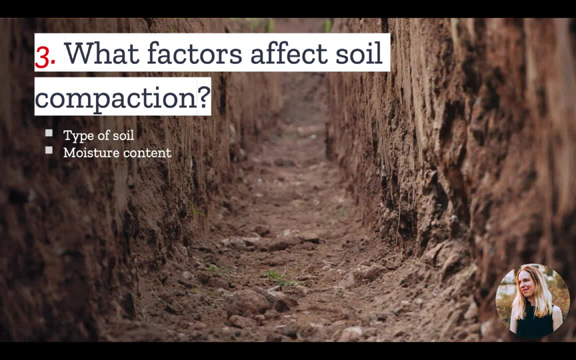 In fact, the maximum soil dry density is only achieved when the water content is at its ideal level. There are also several other factors that affect soil compaction, including the type of compactor you use. the thickness of any layers of soil you are adding the contact pressure between 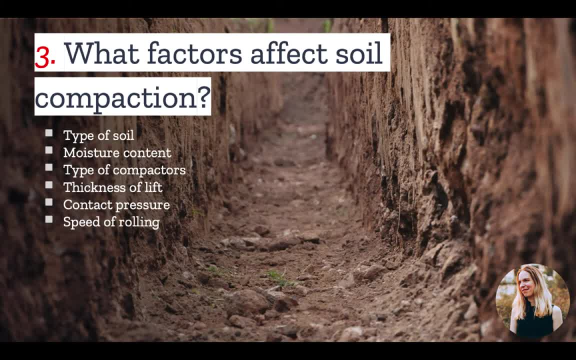 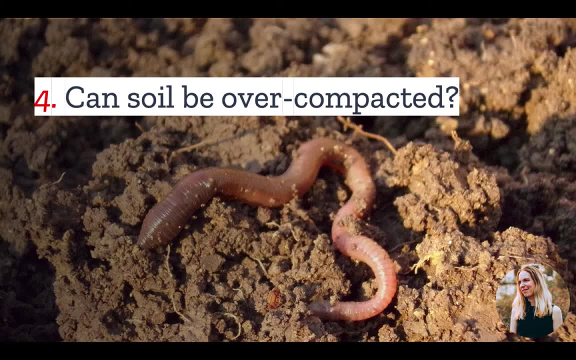 the compactor and the soil, the speed at which you roll over the soil to compact it and the number of roller passes used. Number four: why is soil compaction important? Well, highly compact soils. we've covered why soil compaction is important, but is it possible to have too much of a good thing? 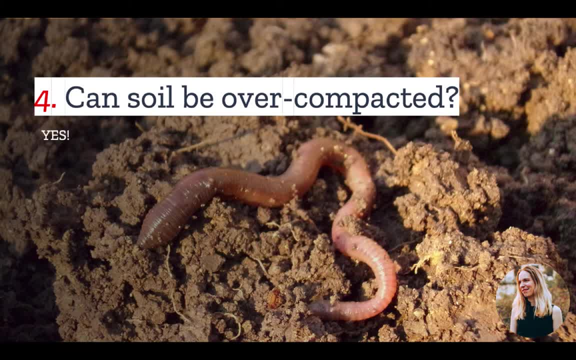 Well, the answer, as is usually the case, is yes, you can overcompact soil. The problem with overly compacted soil is that it makes it difficult to grow plants, But fortunately, there are a few things you can do to help overly compacted soil recover. The best way to handle overcompaction. 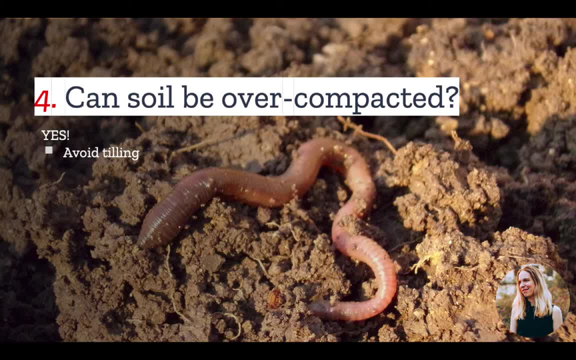 is to avoid tilling your soil when it's too wet or dry or, even better, if you're using a compacted soil, avoid tilling it altogether. In addition, there are some things you can do to help loosen compacted soil, including using an aerator, working in organic materials and adding earthworms. 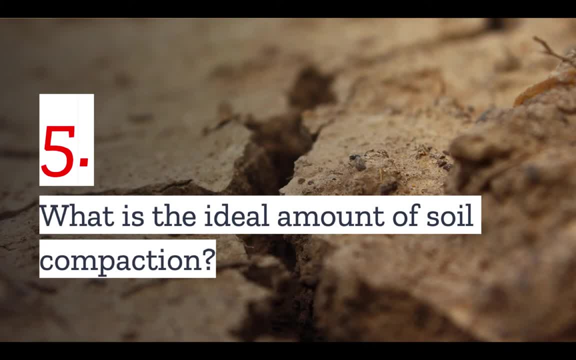 Number five: if both over and under compaction are bad, what is the ideal amount? You'll often hear 95% soil compaction as the target compaction threshold to ensure that construction projects are erected on a solid platform. This means that soil compaction is not as good as it used to be. 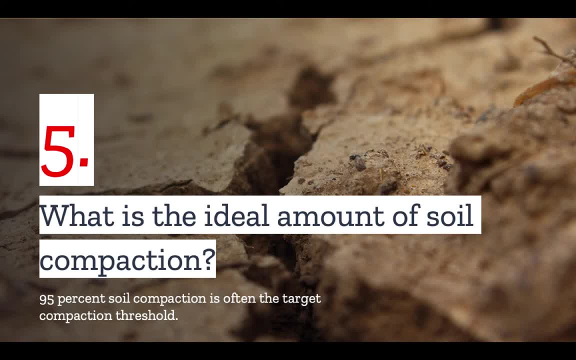 So if you're using a compacted soil, you'll often hear 95% soil compaction as the target compaction threshold to ensure that construction projects are erected on a solid platform. This means that the soil has been compacted to 95% of its possible density through compacted efforts. However, 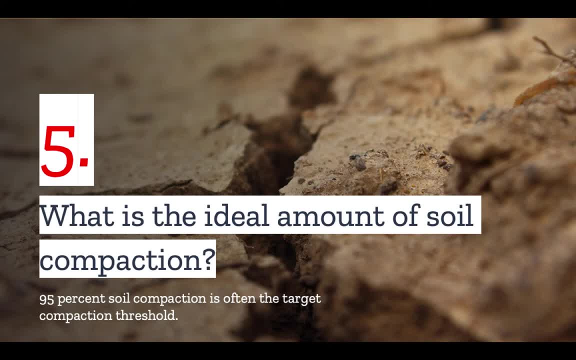 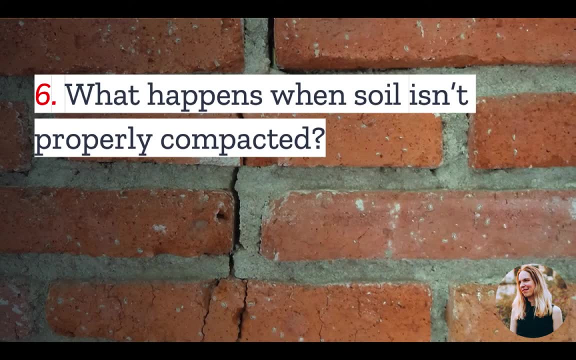 in general, the design engineer will determine the compacted threshold required for your project based on an analysis and testing of your land soil. And number six, what happens when soil is not properly compacted? Well, as we mentioned, the primary concern with poorly compacted soil is soil settlement And settling soil. 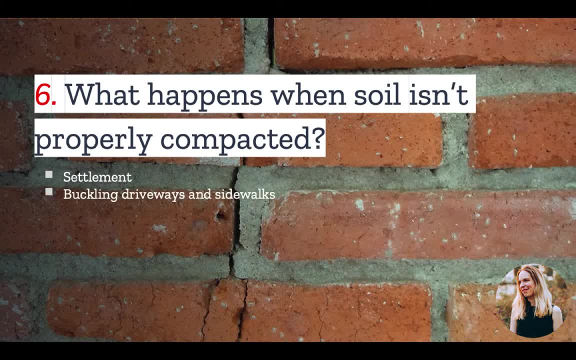 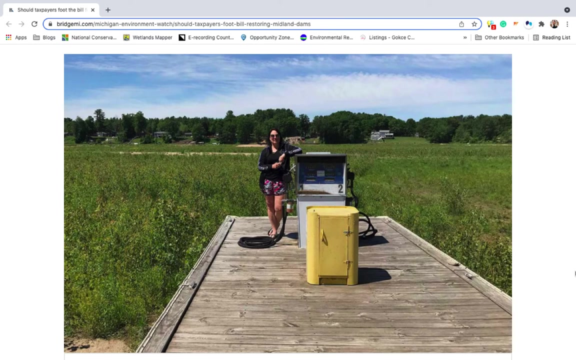 causes a number of issues, including buckling driveways and sidewalks, cracks in foundations and structural walls, ponding and flooding, or overall poor drainage on the land And, in worst-case scenarios, poorly compacted soils can even cause structural failures. Which brings us back to Linda and the Edenville Dam. On May 17, 2020,, Linda watched the rain start. 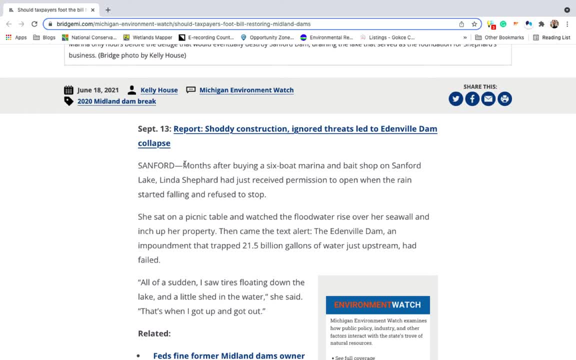 with little more than a shrug. Michiganians are a hardy lot, and especially when it comes to soil management. The spate of spring rain was not about to stop Linda- not when she had just received permission to open her bait and tackle shop. So Linda stayed open and she continued to do so. 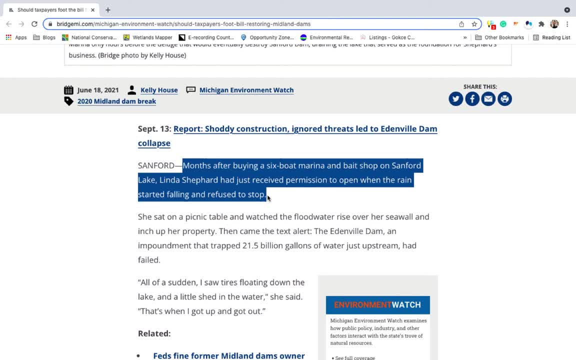 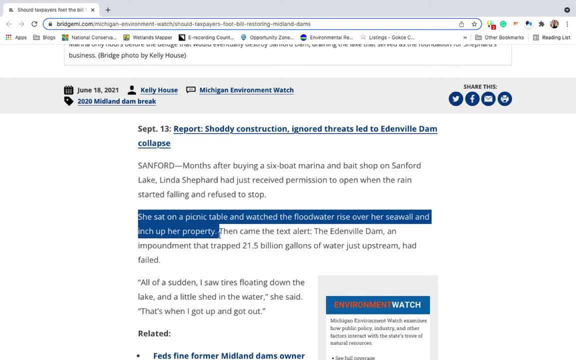 over the next two days as the rains continued and the Titawabasa River began to flood At 5.46 pm on May 19,. she was sitting at a picnic table watching Sanford Lake swell and rise over her seawall. Her phone buzzed and she glanced down at the emergency alarm. All Midland City residents, it said, need to evacuate due to dam collapse. On that eventful May day, the Edenville Dam was just shy of 100 years old. Built in 1924,. the Earthen Embankment Dam holds back the Titawabasa River in central Michigan. 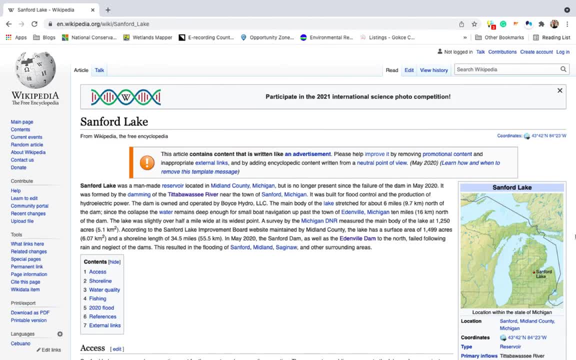 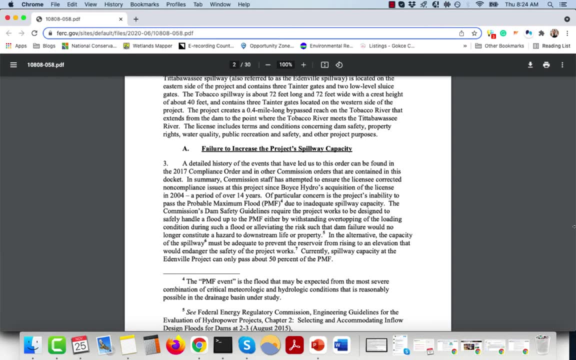 Just downriver is the Sanford Dam, which forms Sanford Lake, the lake upon which Linda's shop sits. The Edenville Dam was not in good shape when the May rains hit. Yet the May rains hit and the Edenville Dam was still in good shape. 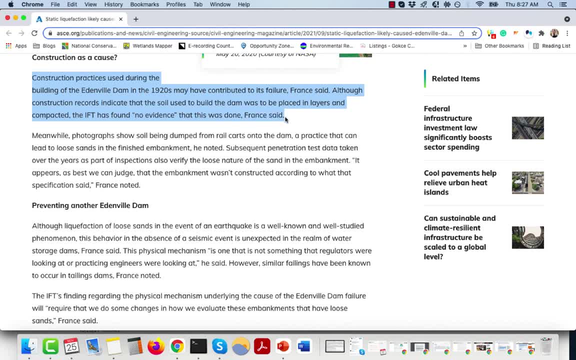 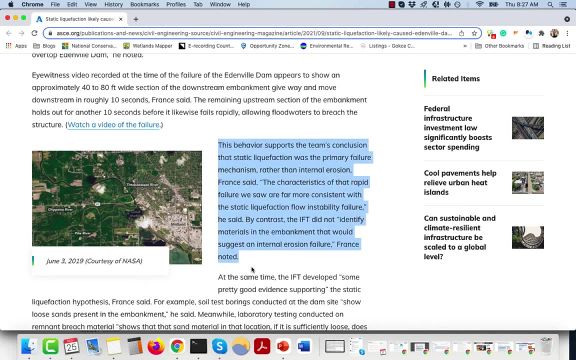 The dam was built before modern principles of geotechnical engineering, so the sand that composed the dam's walls was simply dumped in place and left uncompacted. Thus, when the heavy rains hit, the buildup of the water pressure against the dam walls caused the uncompacted. 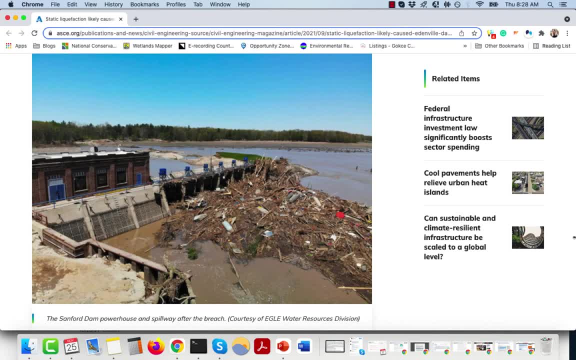 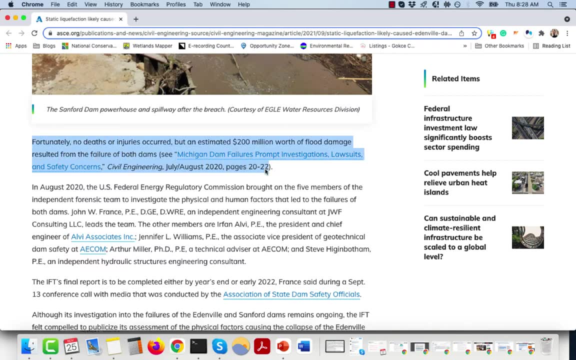 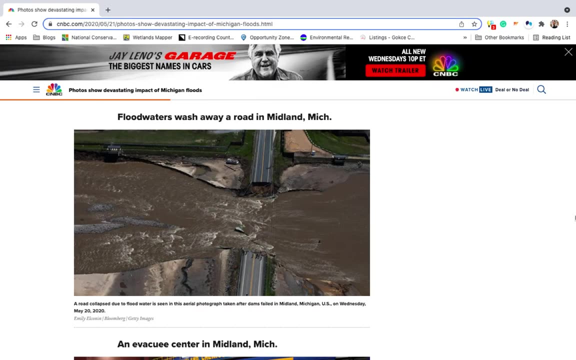 sand to liquefy, The Edenville Dam failed, flooding the river and overtopping the Sanford Dam, causing it to fail as well. Over 2,500 homes and buildings were flooded, causing over 200 million in damages, which is why you never want to cut corners on things like proper soil compaction. 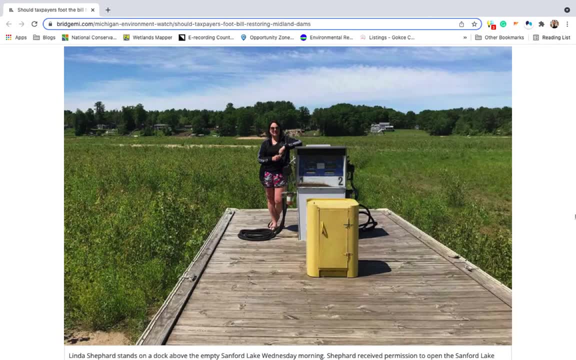 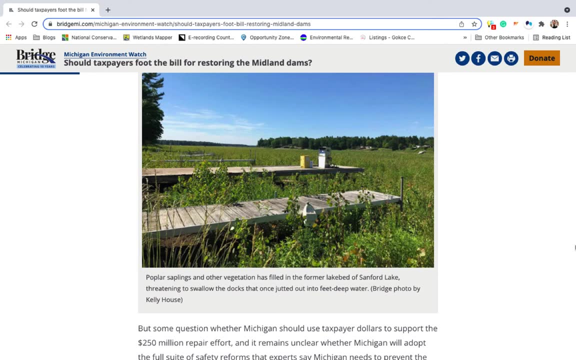 But if you're wondering what happened to Linda, she has not rebuilt. Why do so when Lake Sanford no longer exists? In its place is a grove of poplar, raising a whole new set of thorny questions about whether the dam should be rebuilt.